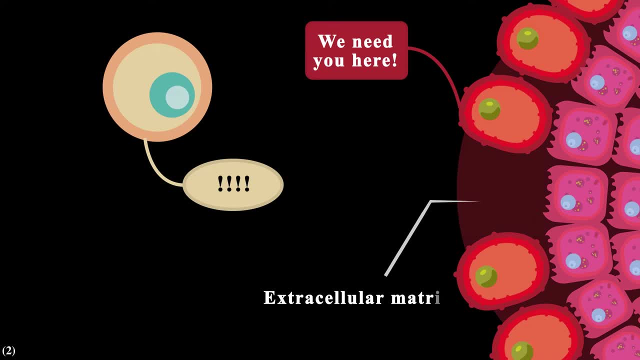 Often, a non-cellular structure can be found in our tissues, which we call extracellular matrix or ECM. The extracellular matrix has a very complex structure made of different components. Okay, wait. In my previous videos I told you that the difference between scarring and regeneration 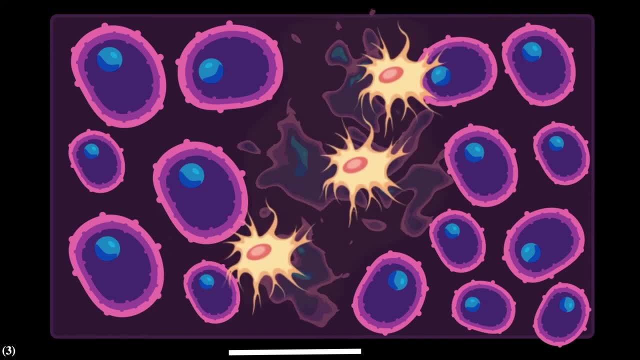 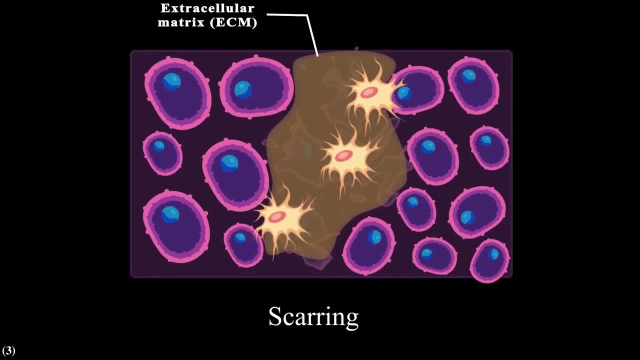 is that in scarring, fibroblasts can be activated to produce extracellular matrix to the wound and make scar tissue. But that was just an oversimplification. In a less simplified way, fibroblasts activate in both scarring and regeneration. but the composition and the 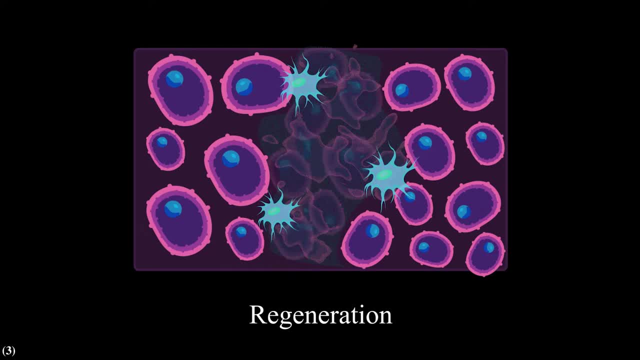 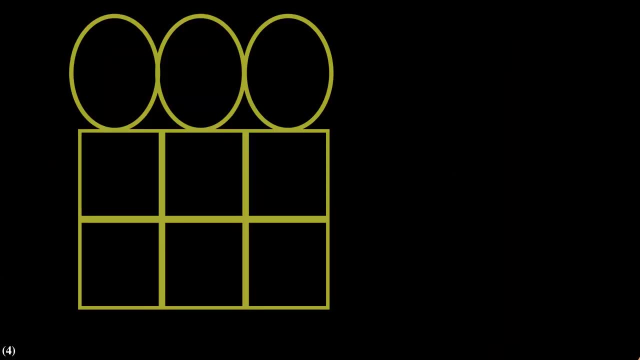 amount of the extracellular matrix in scar and normal tissue is completely different, Which is a very complex topic and we need to talk about in details in different videos. But what is important here is that the extracellular matrix is like a frame of a house for 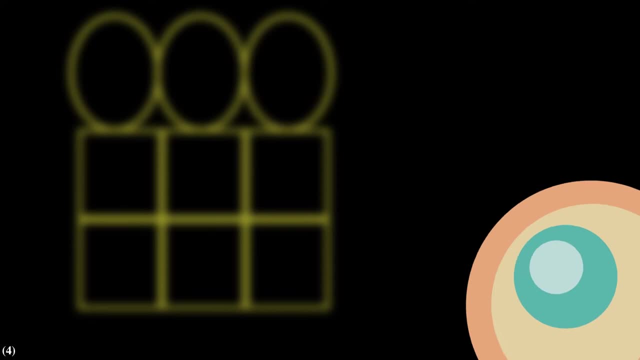 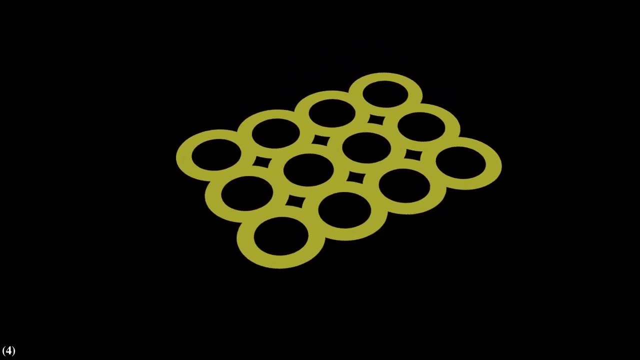 tissues. They hold the instructions for our cells to make specific tissues and organs, Since different houses have different frames, different tissues have different ECM with different composition and structures. But why I'm telling you all this? and what's the role of biomaterials here? 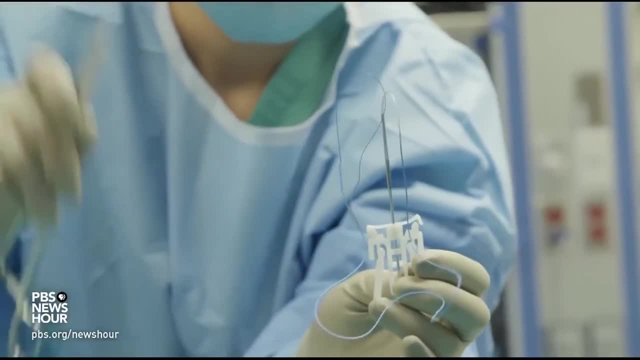 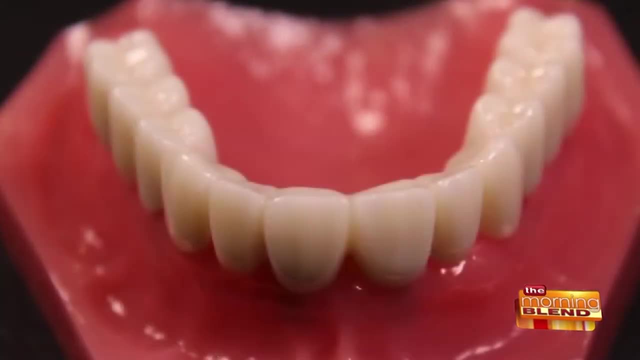 Traditionally, we use biomaterials because of their mechanical functions for use in prosthetic and medical devices such as artificial hips or dental implants, And we tried to pick a material to not interact with the host biological system because we wanted to decrease the chance of 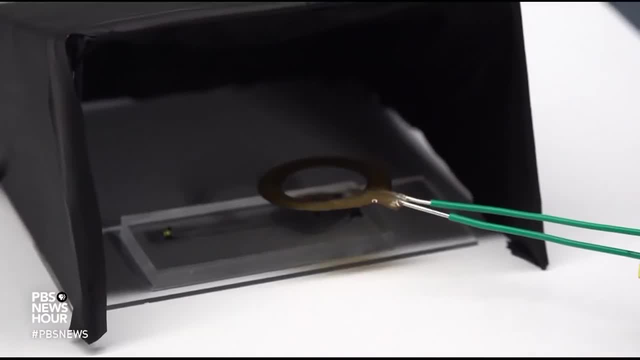 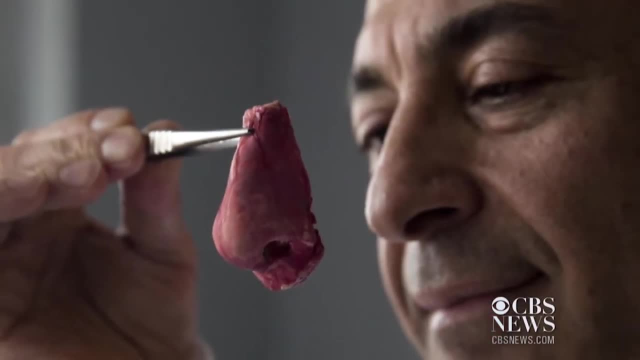 rejections by the host immune system. But now, with improving different technologies, we are able to design biomaterials to mimic the physical and chemical cues that our stem cells need to make specific tissues. But how we can do that and which properties we should pay attention to. 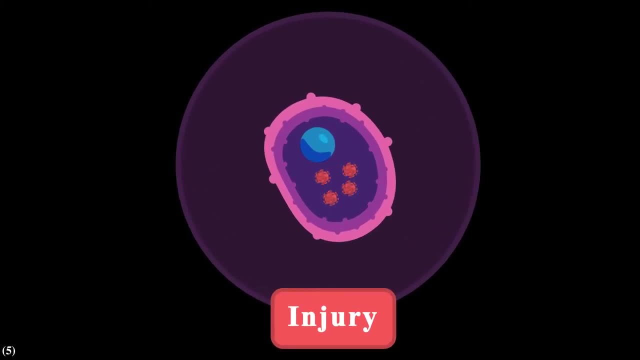 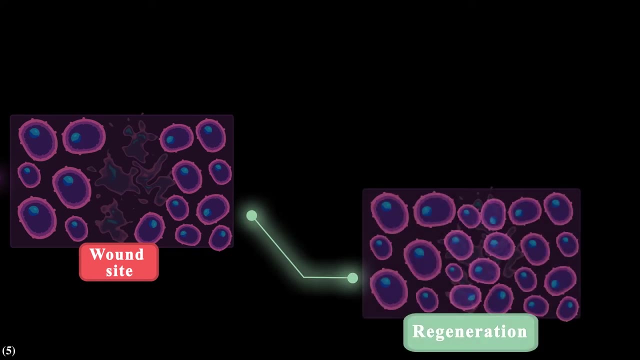 Until now we have been talking about that, if an injury happens in our body, the cells that died in our tissue should replace with new ones, which we call this process regeneration. But, as we talked about it before, we are not good at regeneration and for some reason our body makes scar tissues. 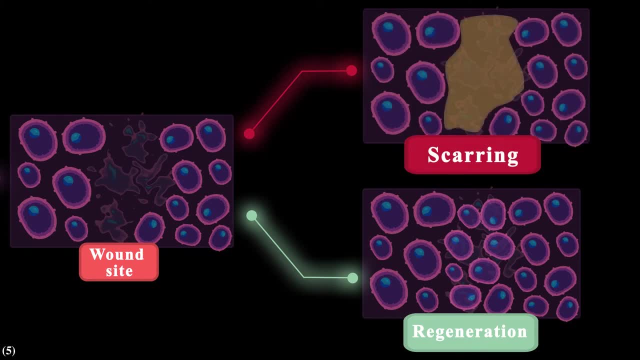 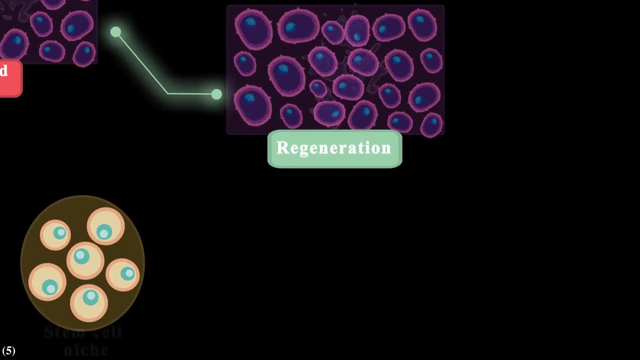 in most injuries, which brings a lot of complications. We know that our specialized cells or fully differentiated cells can divide to make new cells, But we found that most of our tissues have a niche for stem cells which can proliferate to make more of them, and they can. 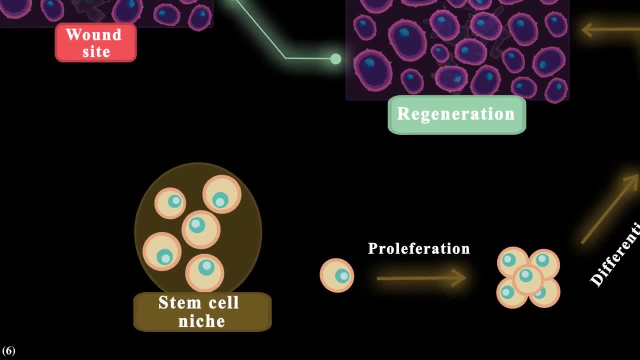 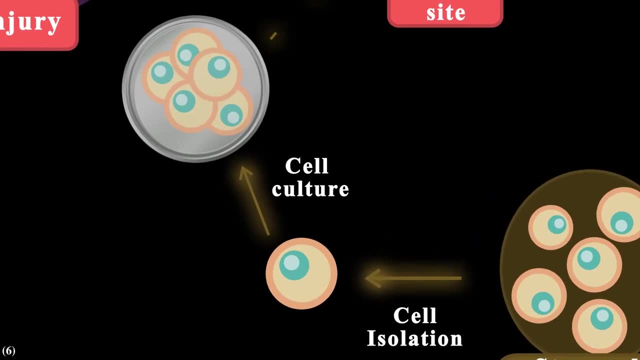 differentiate into specialized cells. We started developing techniques to isolate those stem cells from our tissues and we started culturing them in the lab to make more of them, So we can inject those stem cells directly into the sites of injury, which we call cell transplantation. 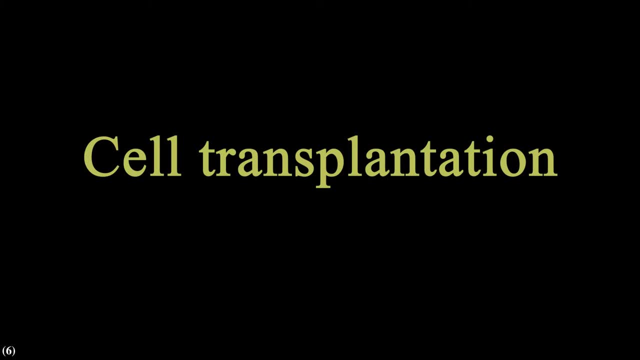 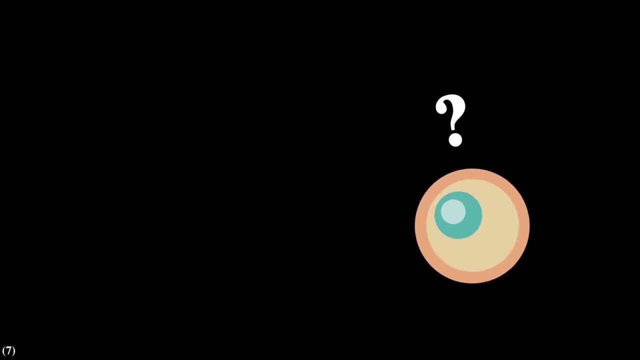 But it doesn't work quite well. Here's why The stem cells need to proliferate and differentiate into cells which are dead during injury, And they need to know the exact position and time to do all of those things. For doing that, they need appropriate instructions, which. 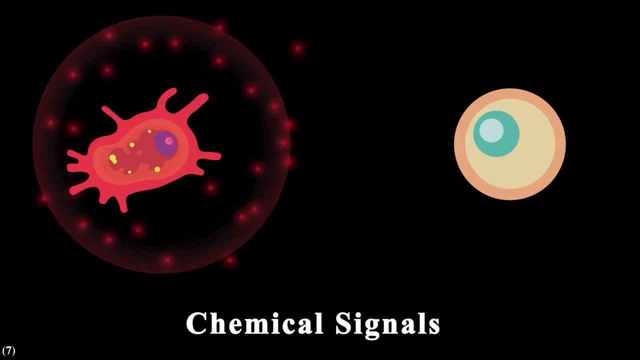 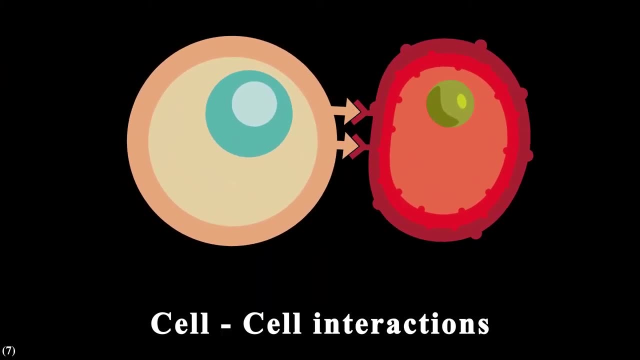 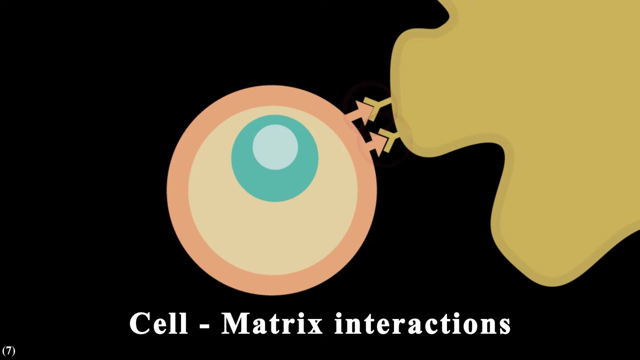 they learn from three factors: The chemical signals which are produced by different cells, such as damaged cells and immune cells. The direct interactions of our cells together, which we call cell-cell interactions. And the other one is the direct interactions of our cells with their extracellular matrix, which we call cell-matrix interaction. 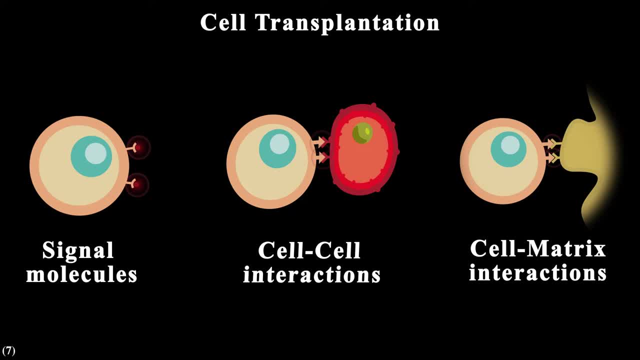 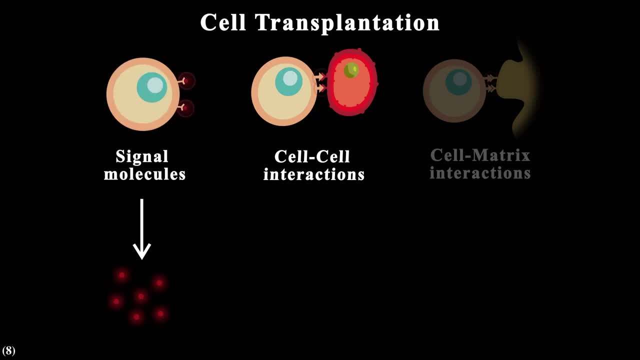 In cell transplantation we have cell-cell interactions but we eliminate signaling molecules and cell-matrix interaction. For solving the signaling part we can add signaling molecules ourselves, And for cell-matrix interaction we can make a temporary substrate for our cells. 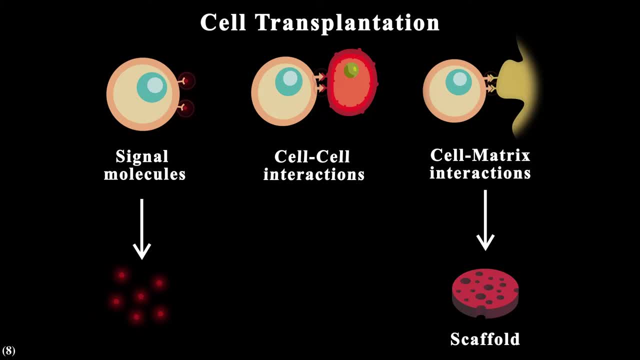 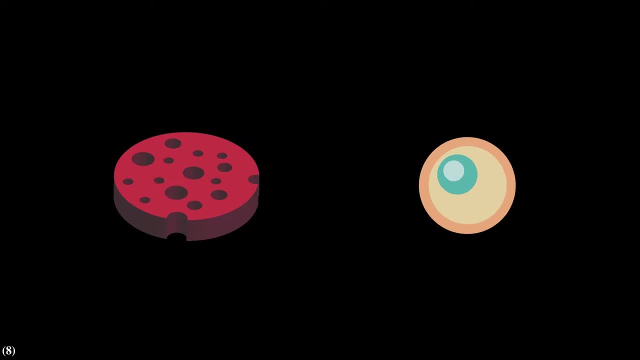 which we call a scaffold, to provide a suitable environment for them. And obviously we use biomaterials to make our scaffold. But not all scaffolds and biomaterials are favorable for our cells. Cells are really strict and picky about their environment. After considering a variety of 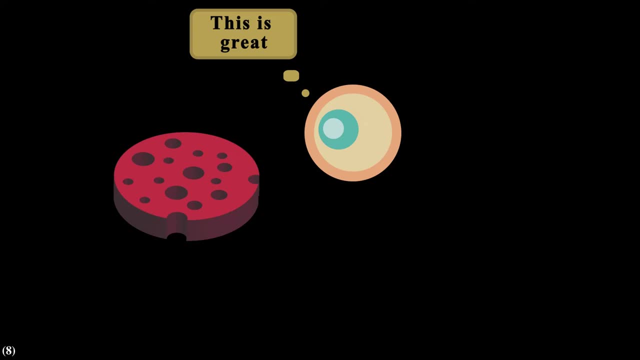 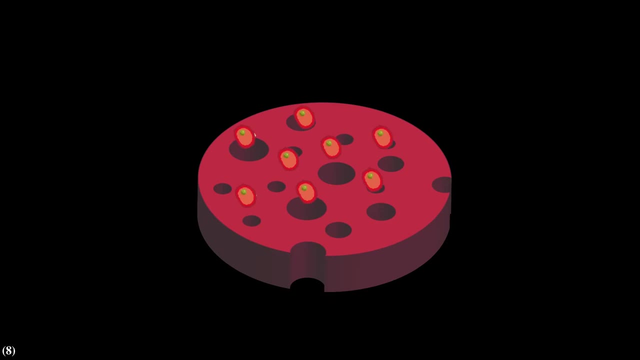 factors, they can change their behaviors. What I mean by behavior is that they can run away or they can move towards and attach to the scaffold. They can proliferate and differentiate into different cells and they can signal to other cells to do the same thing. So what are those? 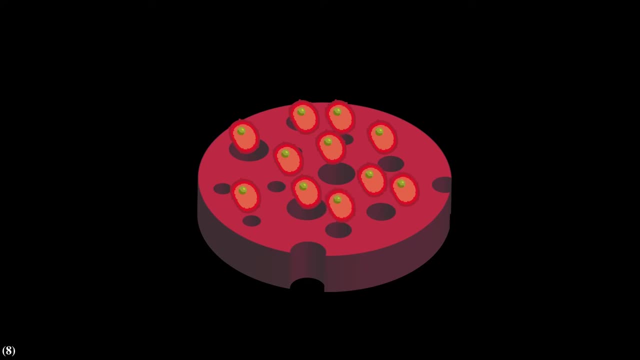 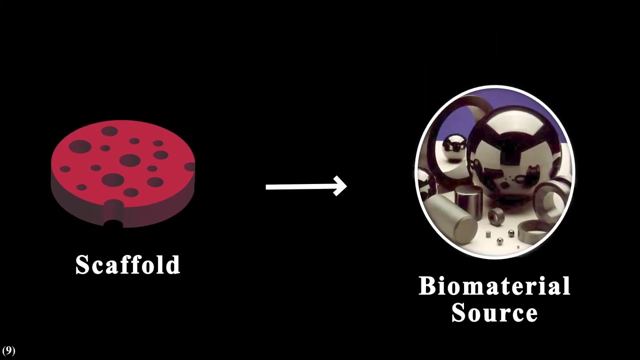 factors and how they can affect the behavior of our cells. Let's imagine that you want to build a scaffold in the lab. First you need to consider which biomaterial you can use. There are a lot of biomaterials and all of them have their own pros and cons. We can extract biomaterials from natural 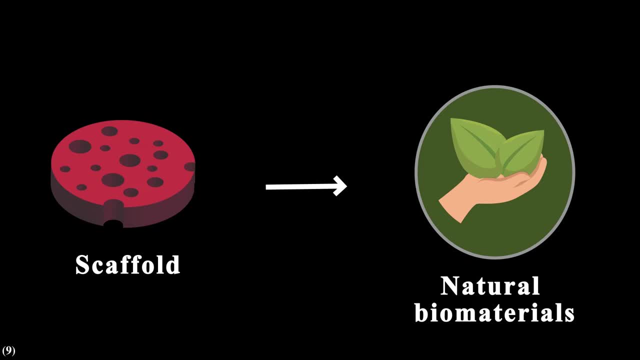 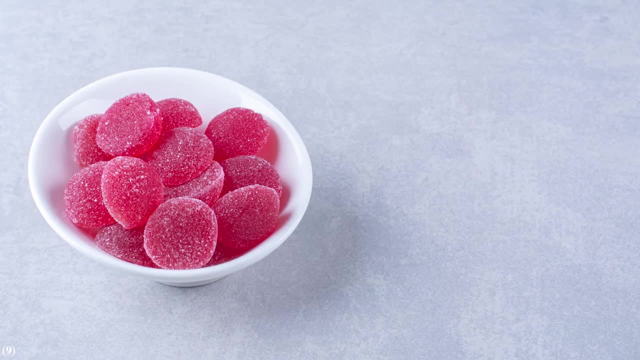 resources like plants, animals or even humans. For example, gelatin is one of those biomaterials which can be extracted from animals like fish, chicken or cattle And, surprisingly, it's the same gelatin that we use as an ingredient in our food. We can use synthetic biomaterials as well. 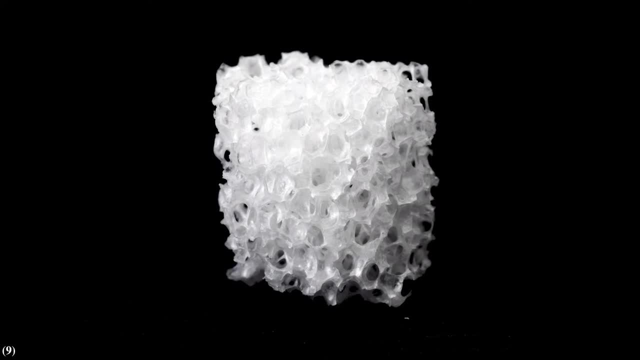 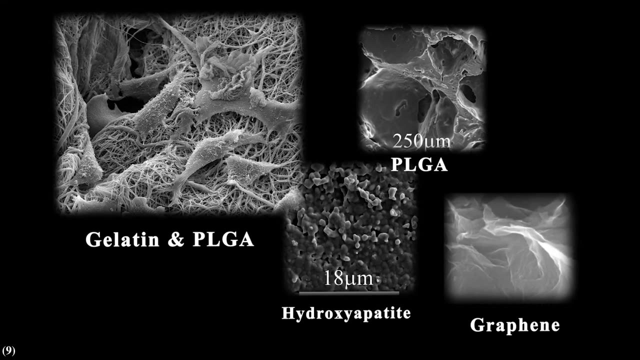 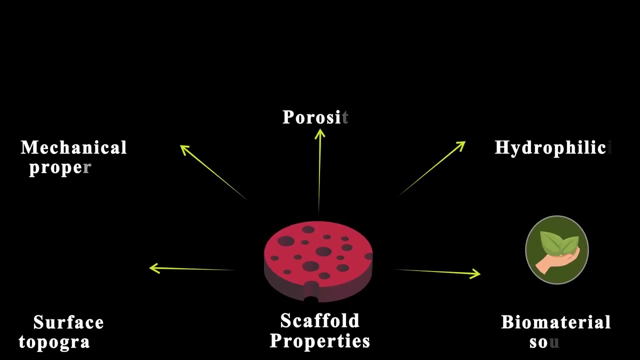 like ceramics or many polymers that we can make in the lab with different chemical techniques. But we should consider that every biomaterial gives your scaffold different properties. At first we need our cells to move towards our biomaterial and attach to it, So we need to pick a hydrophilic biomaterial. Hydrophilic means how much our biomaterials 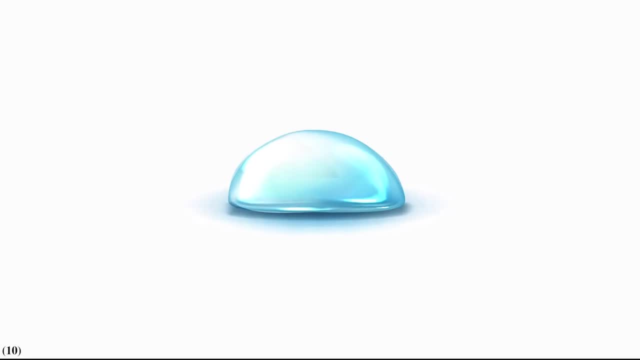 can attract water and we can measure this in the lab by putting a droplet of water on the biomaterial's surface. If it is less than 90 degrees, we consider the biomaterial hydrophilic and our cells love hydrophilic surface. But the attachment of our cells to the surface 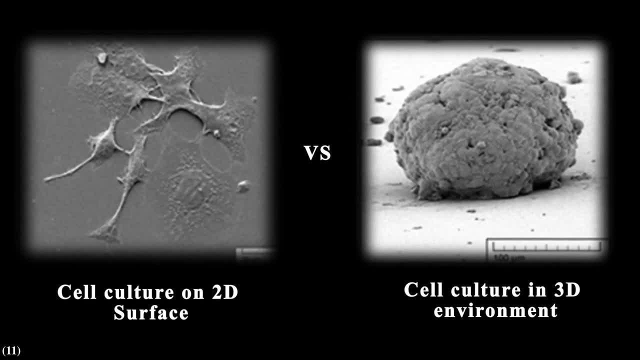 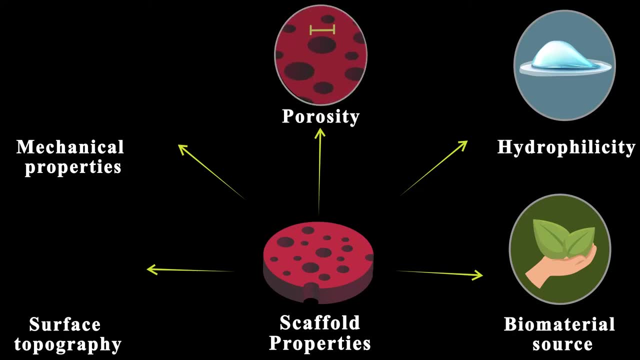 of biomaterials gives them a 2D environment. But the reality is that our tissue and organs have 3D-structures, So we need to design a lot of pores in our biomaterials so our cells can go inside the biomaterials and make 3D-structures, And that's the reason the size of the pores is. 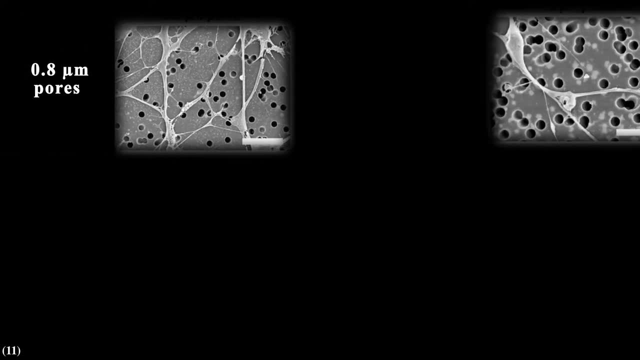 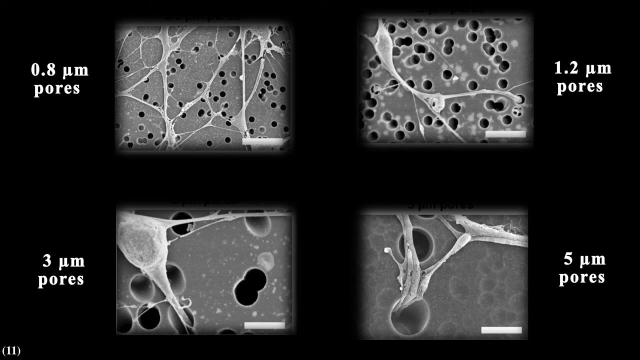 very crucial Because different cells have different sizes, so their desire is different. Some prefer small pores, but others prefer the big ones. Even the number of pores is really important. For example, in a study by Ma and colleagues they found that low porosity about. 1.5%. So in the lab we have a low porosity of about 0.6% And we found that it's a lot lighter than the size of the pores, because the pores are less visible, So it's a lot longer And we 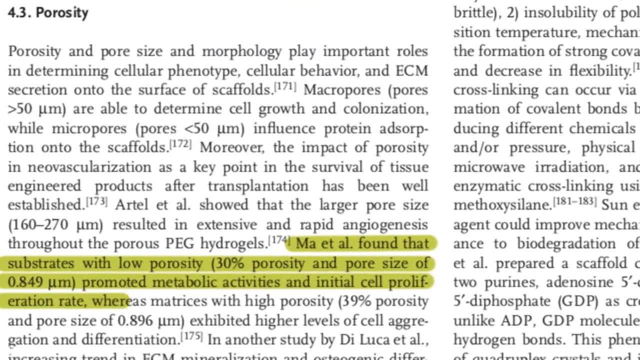 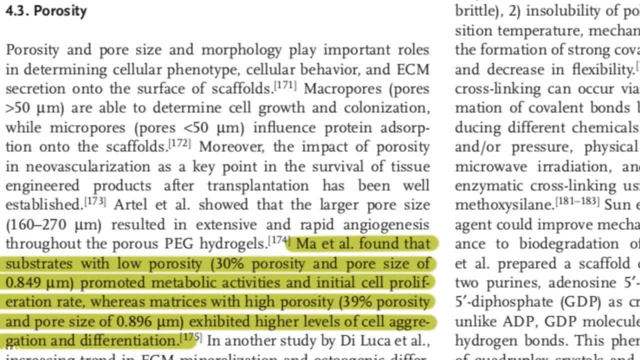 can measure the size of the pores by measuring the size of the pores, But we have to take care of it. with a size of 0.84 micrometers can promote metabolic activity and the rate of cell proliferation, but 39-porosity with a size of 0.9 micrometer showed higher level of cell aggregation and 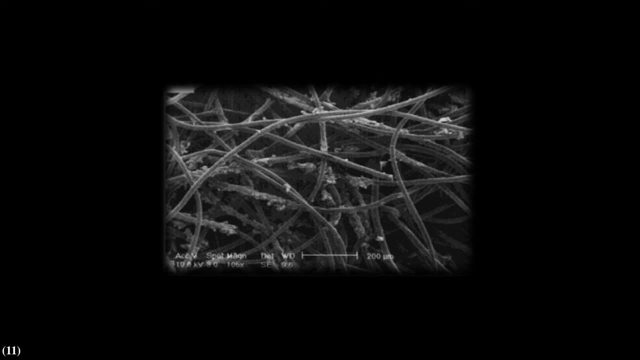 differentiation. This is a picture of a biomaterial that was taken by scanning electron microscopy or SEM, which I'm not going through the details, but it's suffice to say that you can see the fibrous structures of the biomaterial and actually you can see the cells in here. 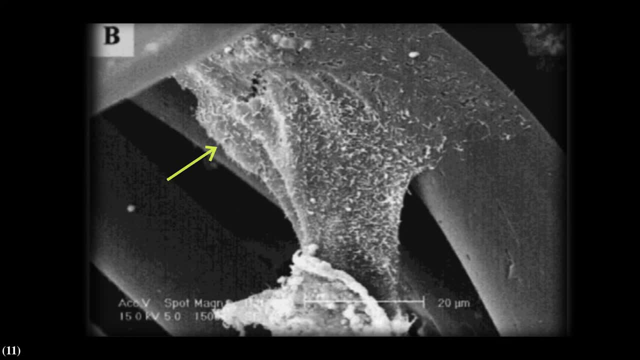 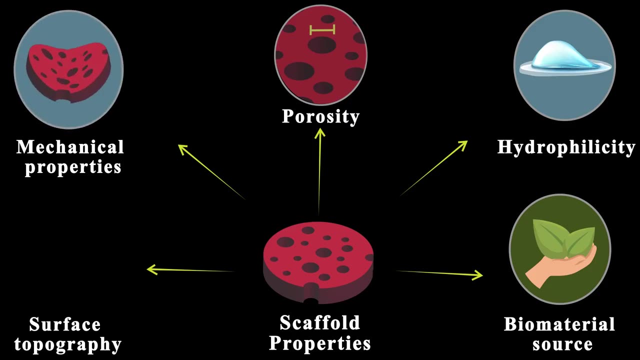 Let me zoom a little bit. You can see this cell is completely attached to the biomaterial and is happy like really happy. If you want to design a biomaterial, its mechanical properties are very important. The mechanical properties of every tissue are different and it guides shape, morphology.